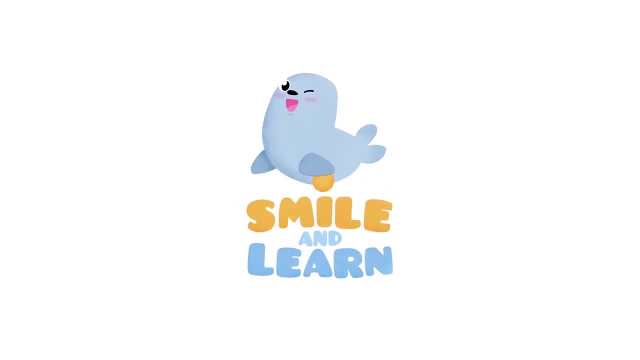 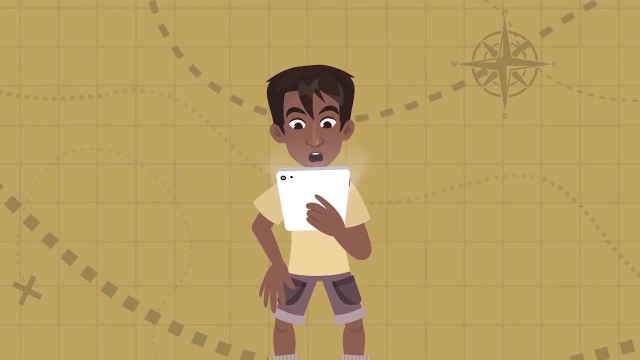 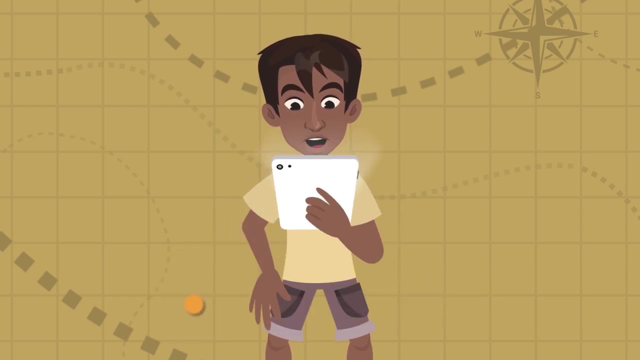 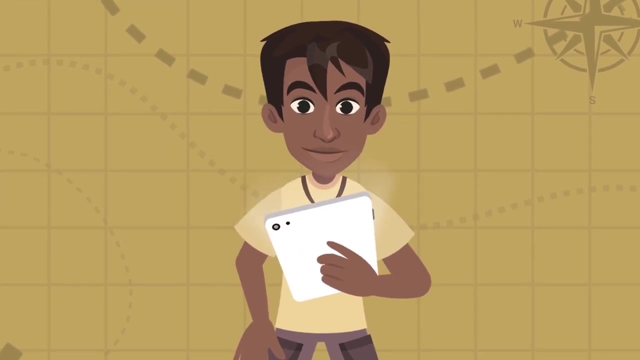 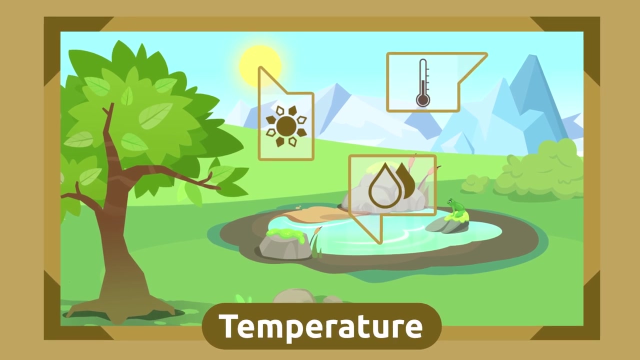 Hello friends, Today we're going to discover other places where living beings live. These places are known as habitats. Did you know that We call a habitat a place that has the necessary resources so that living beings can survive? These resources are the light, the water, the temperature, the ground and the oxygen. 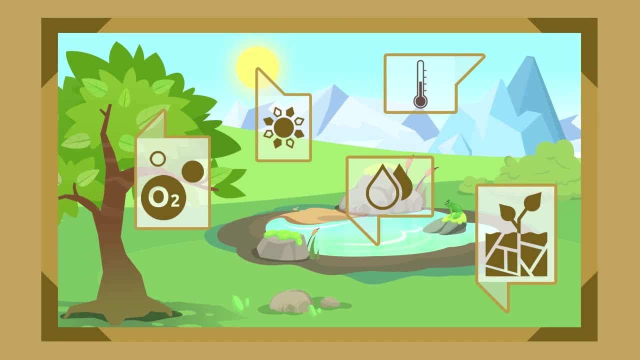 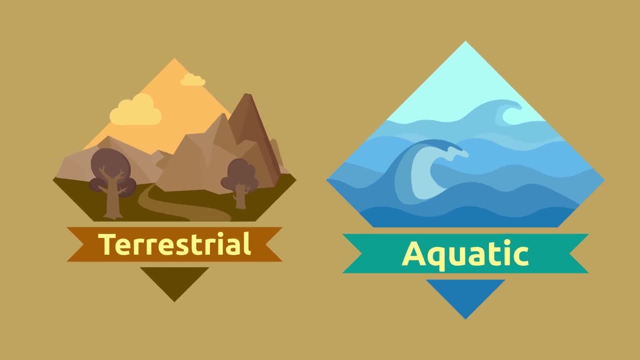 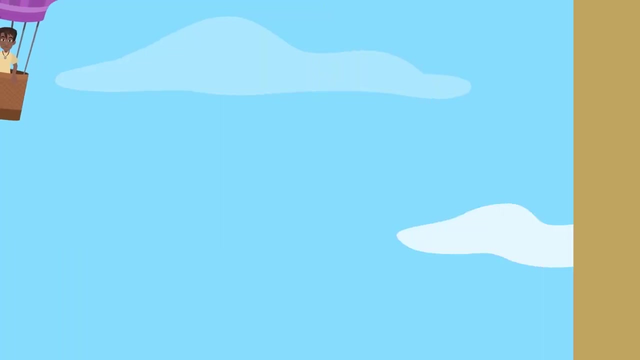 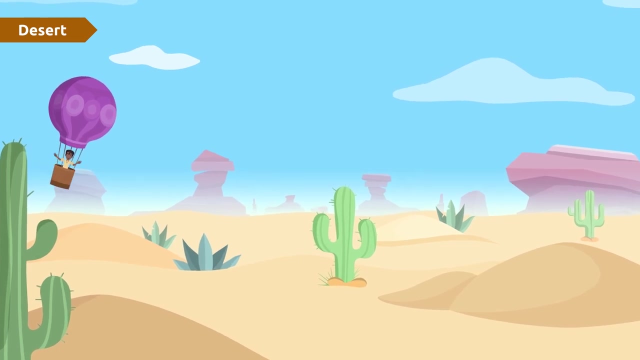 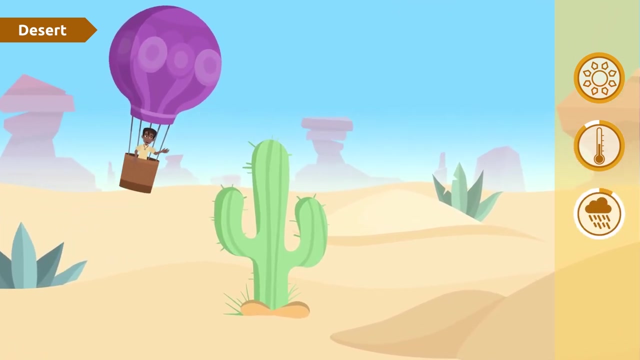 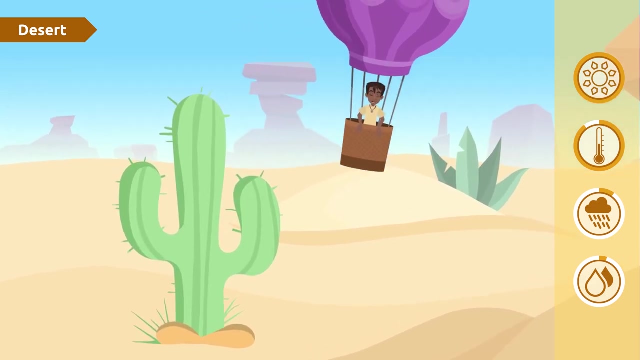 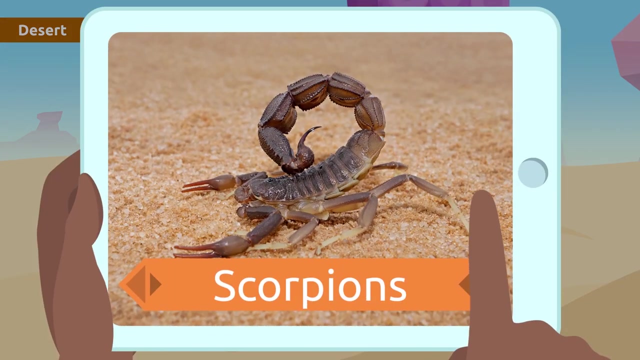 Depending on what these resources are, we can find very different habitats. There are two types of natural habitats: terrestrial and aquatic. Today I'm going to travel to the terrestrial habitats. Are you coming with me? Let's go. Snakes or mammals like camels or dromedaries can live in the desert. 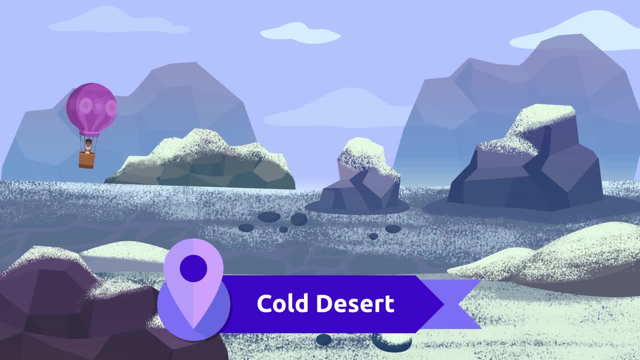 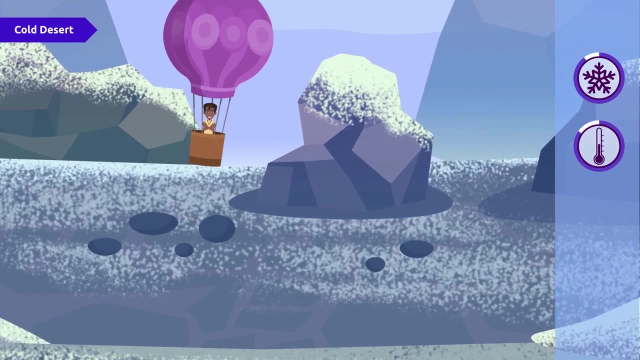 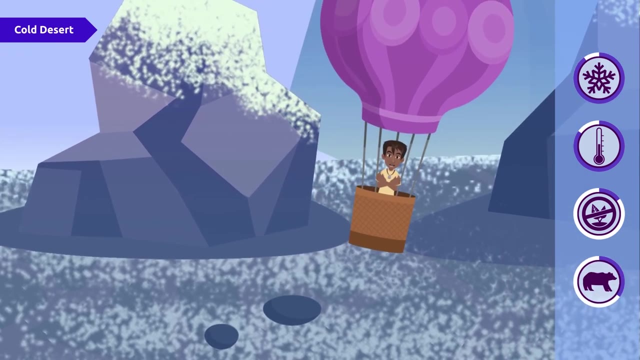 Did you know that there are cold deserts too? Here, everything is frozen and temperatures are extremely cold. There are barely any plants in these habitats. However, we are able to find some animals that have adapted to be able to live in them. 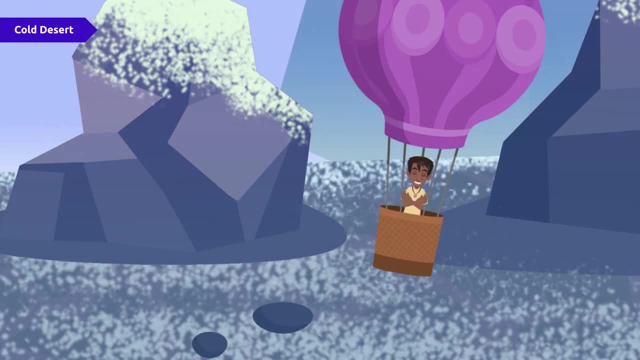 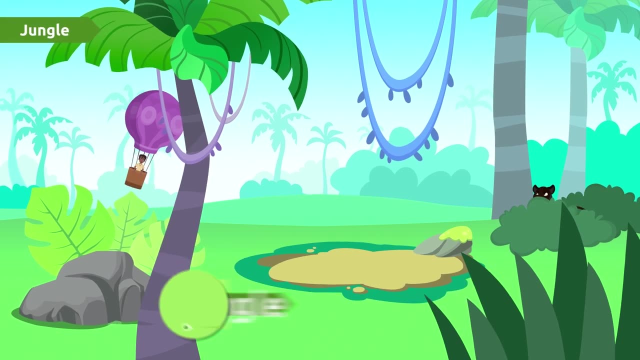 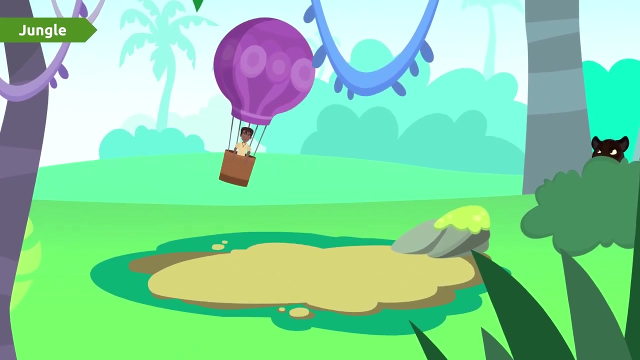 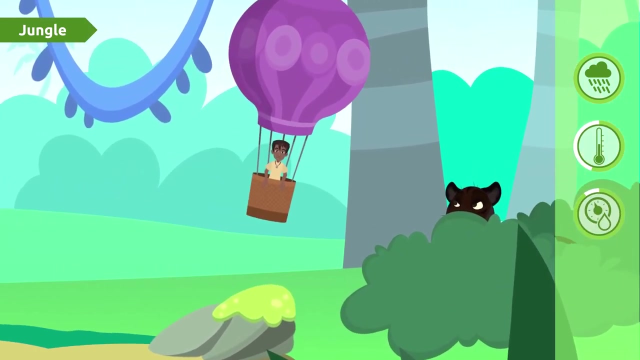 like the polar bear Jungle. We continue our trip. Look how many plants there are. This habitat is the jungle. Here there's lots of rain and temperatures are mild or warm. This favors a humid environment in which there are many living beings. 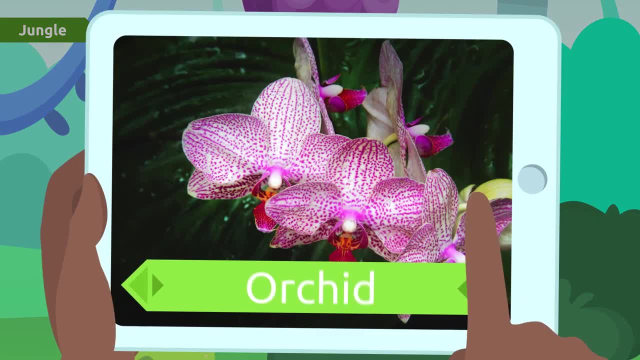 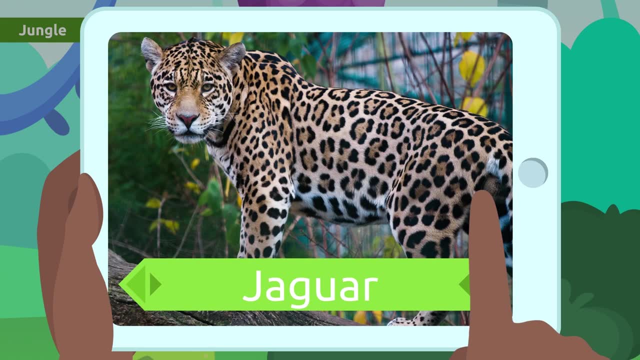 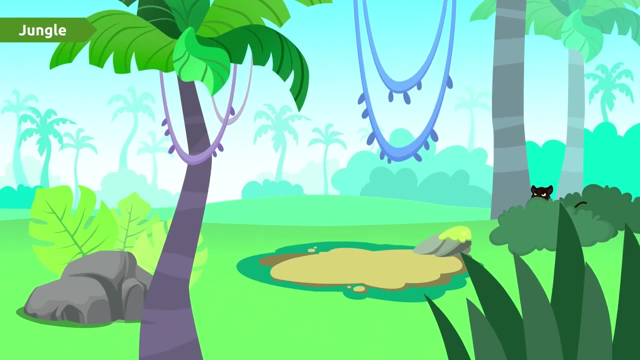 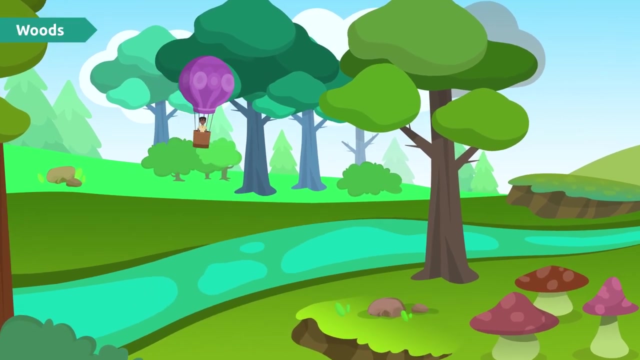 Let's see which ones we can find here. Look, an orchid And a hummingbird. This can be a panther or a jaguar. I think I'm leaving. I don't want to be his dinner Woods. We're in the woods. 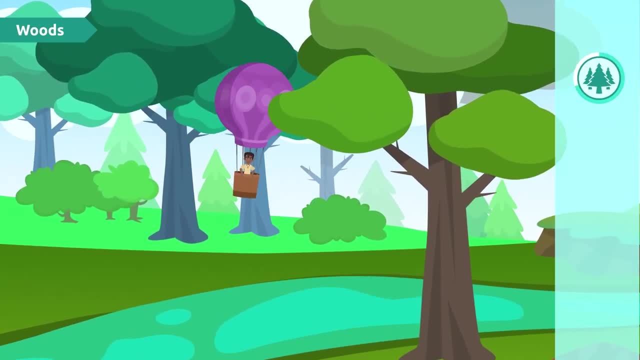 Here too, there is plenty of vegetation, Mainly trees like beech trees or pine trees. Here too, there is plenty of vegetation, Mainly trees like beech trees or pine trees, And shrubs or bushes like the rock rose or the arbutus. 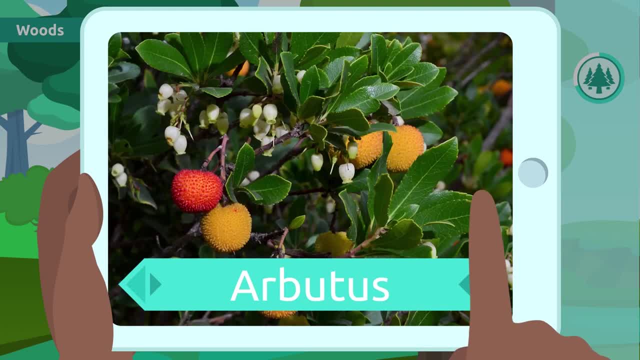 And shrubs or bushes like the rock rose or the arbutus. And shrubs or bushes like the rock rose or the arbutus. Did you know that there are many types of woodlands? Did you know that there are many types of woodlands? 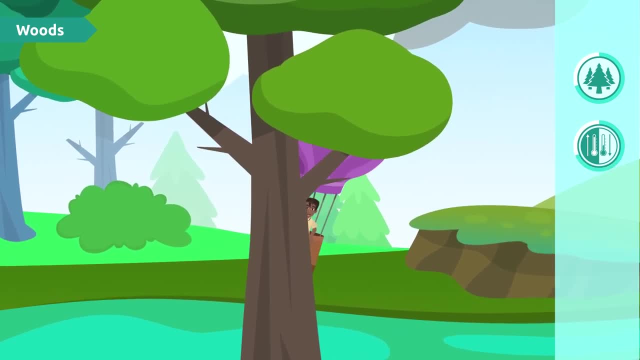 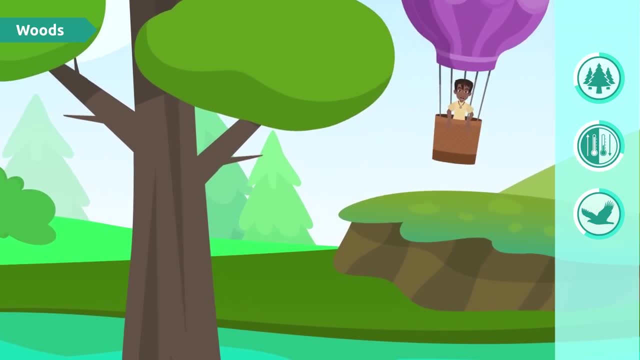 Their temperature may vary from cold to warm and because of this the vegetation and the animals we find there change. In the woods we can find some animals like bears or eagles. In the woods, we can find some animals like bears or eagles. 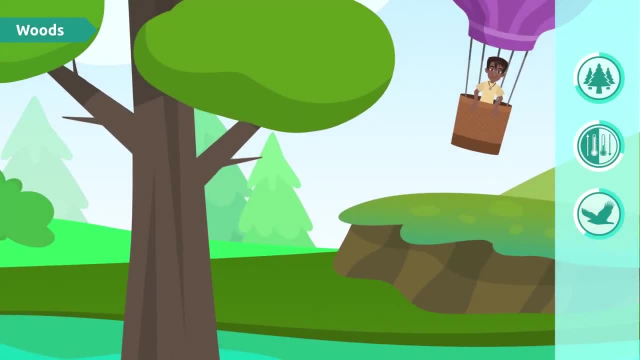 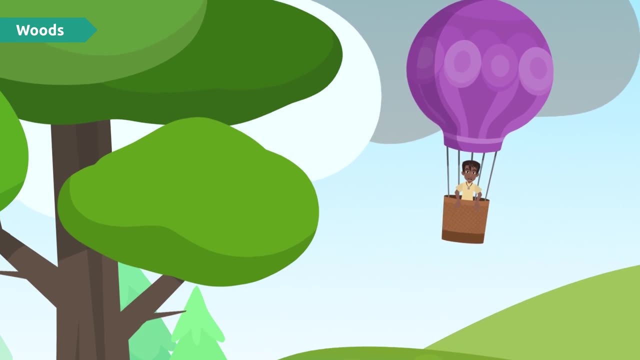 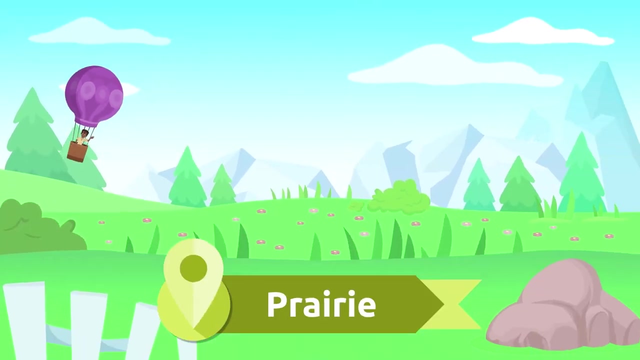 In the woods we can find some animals like bears or eagles. Here too, it rains often. I think that this cloud means a storm is coming. I think that this cloud means a storm is coming. Let's continue our trip Here. we found a prairie. 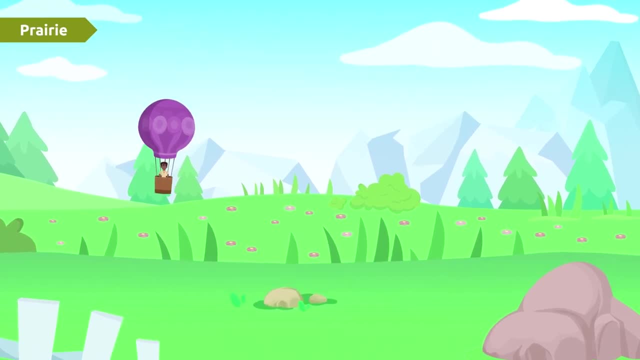 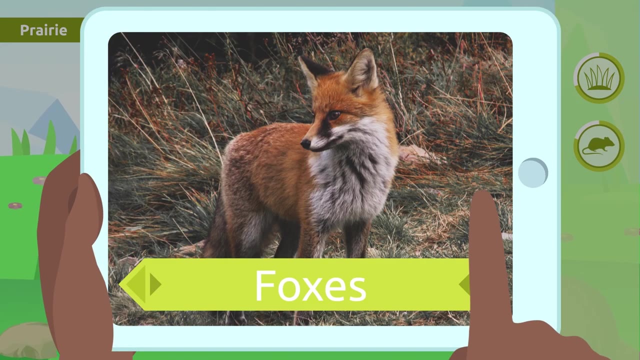 Here we found a prairie. We've just arrived at a prairie. This habitat is characterized by small plants like grass. This habitat is characterized by small plants like grass and animals like foxes, Cauliflower and walnuts. The climate in the prairie is humid. Winters are cold and summers are warm. Savannah. Another habitat with little vegetation is the savannah. Savannas are usually dry areas where it rains very little. However, we distinguish two periods: a dry season with low temperatures, and a season that rains a lot, with warm temperatures. 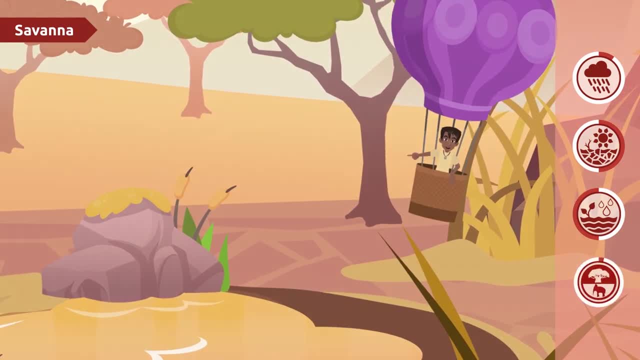 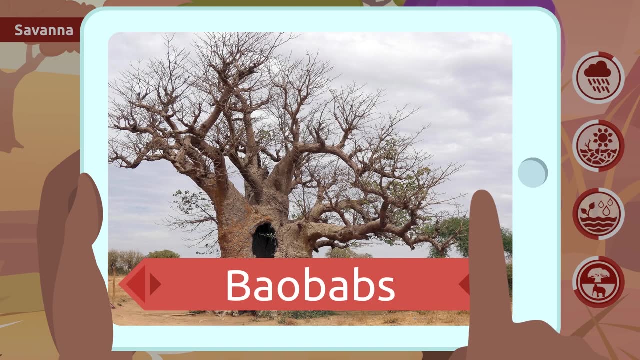 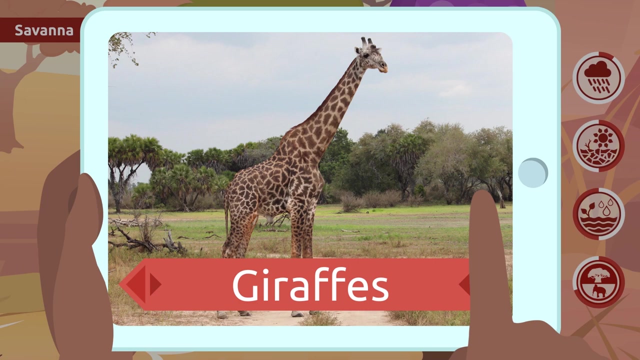 The latter one is called the humid season. Here we can find grass, herbs, non-woody plants and some trees like baobabs. Among the animals, we find many herbivores like elephants, zebras or giraffes. There are also carnivorous animals like lions. 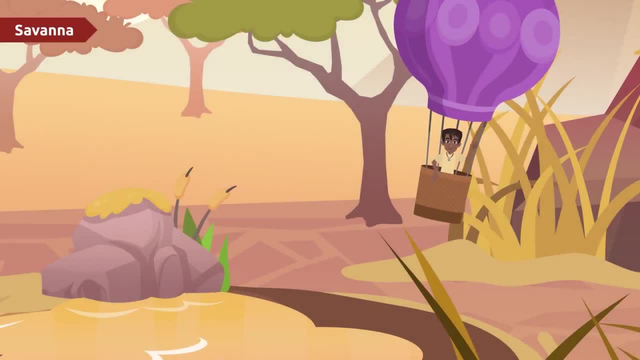 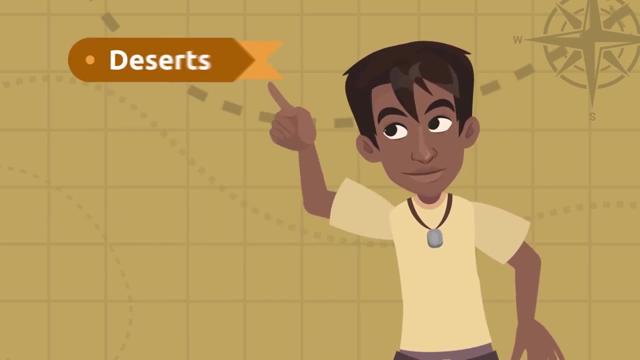 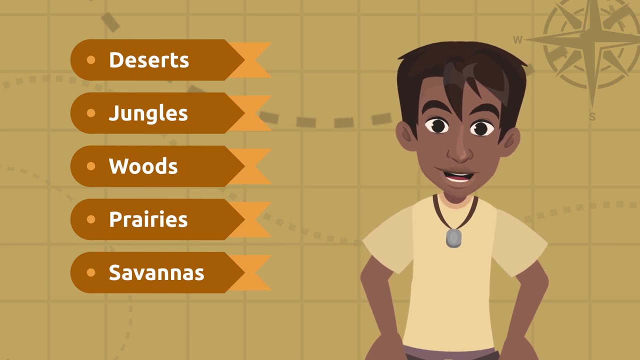 or cheetahs. Today we have seen the terrestrial habitats, among which we find deserts, jungles, woods, prairies and savannas, But we still have aquatic habitats left to visit. Don't miss the next video. 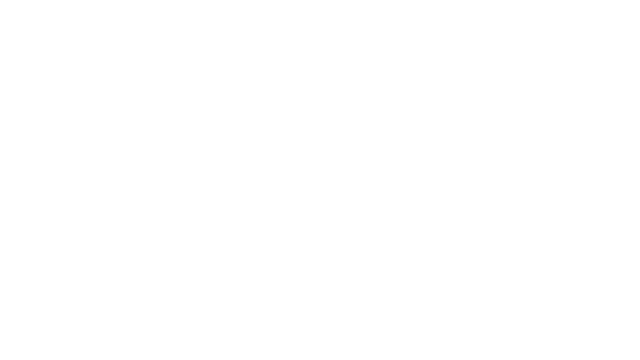 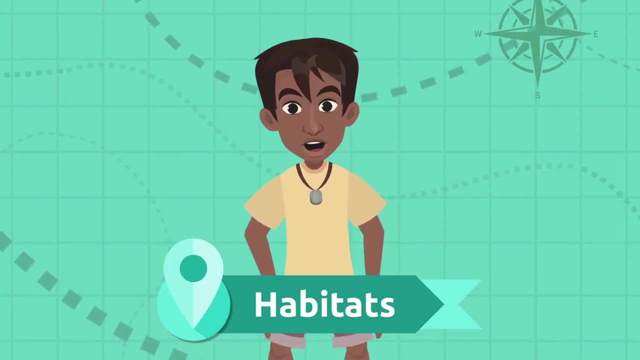 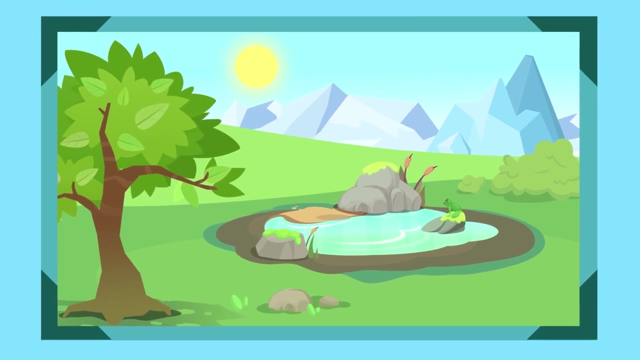 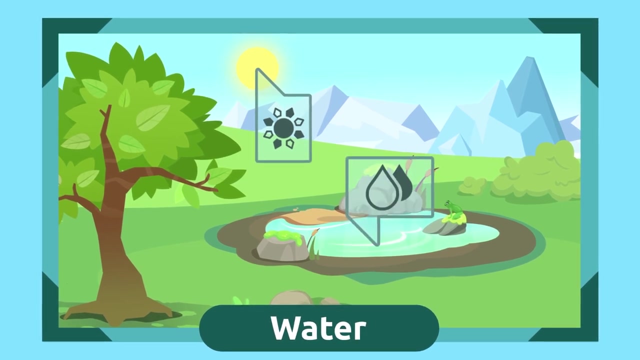 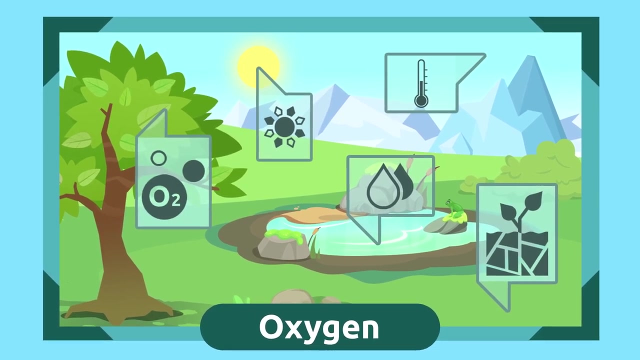 See you soon. Hello again, friends. In the previous video we talked about habitats. Do you remember what they are? We call a habitat a place that has the necessary resources so that living beings can survive. These resources are the light, the water, the temperature, the ground and the oxygen. 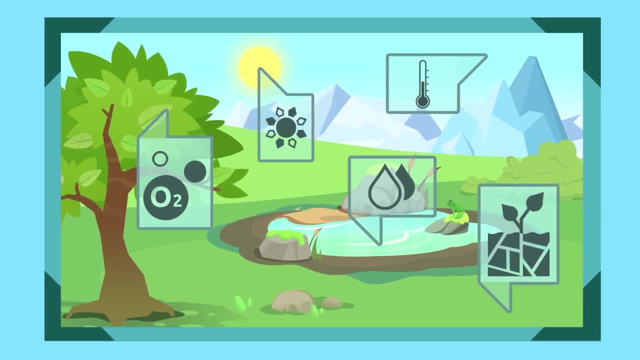 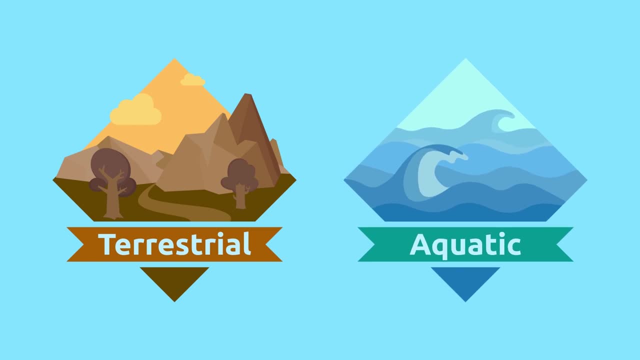 Depending on what these resources are, we can find very different habitats: Fauna, aquatic, Animalsstyles. There are two types of natural habitats: terrestrial and aquatic. In the previous video, we travelled over terrestrial habitats. Today, we will be visiting aquatic habitats. 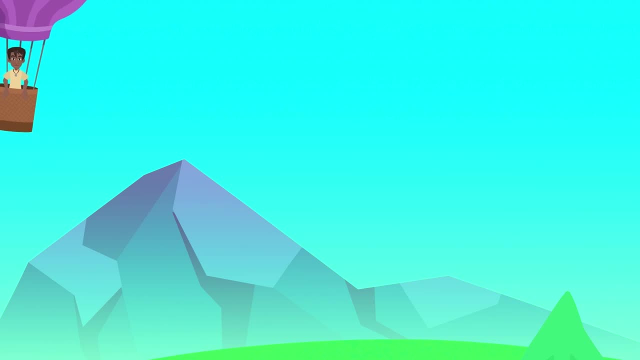 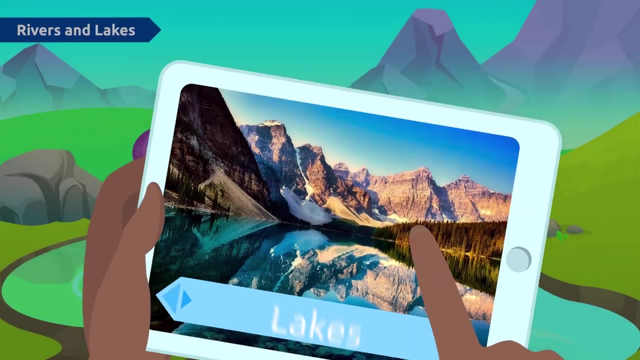 Are you coming with us? Come with us. Rivers and lakes. Rivers and lakes are freshwater habitats. There we can find many other animals, among which fish, lake and fish. Let's Ready Where more are Lake and Rivers. Fr melhores Resort. 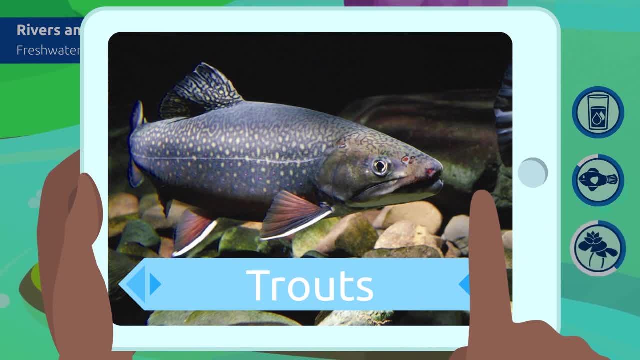 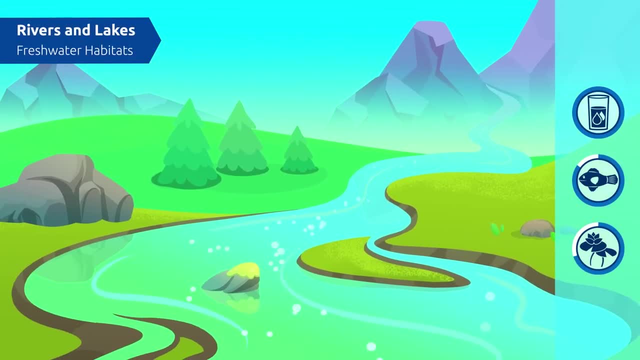 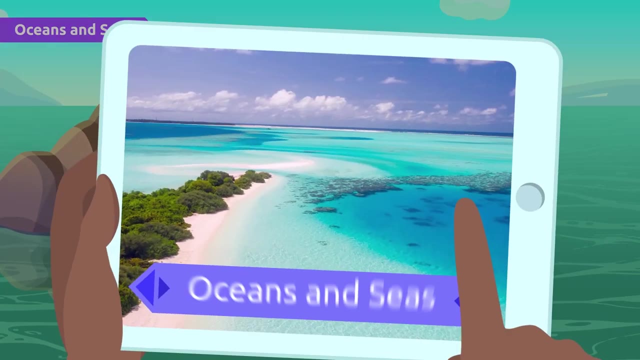 How There are two types Natural Hazards. In the previous videos we Mexico, where we visited river retour. Today, we will be visiting aquatic habitats. Are you coming with us? Rivers and lakes? Are you coming with us? trouts, small plants like water lilies also grow there. oceans and seas- oceans. 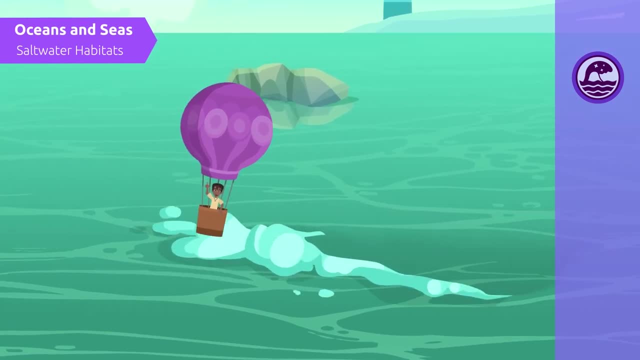 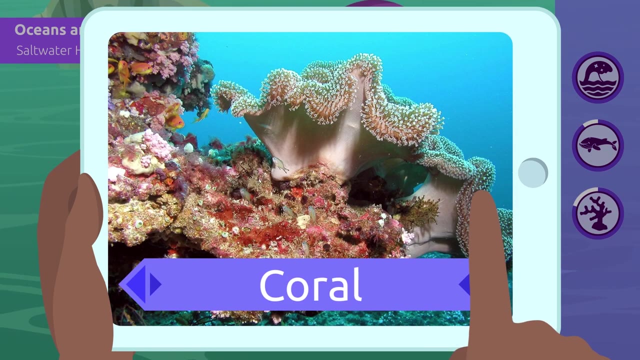 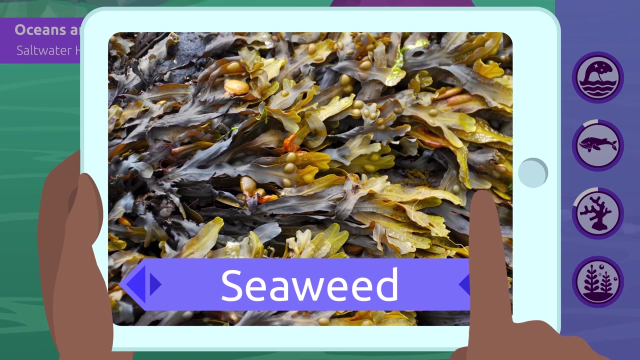 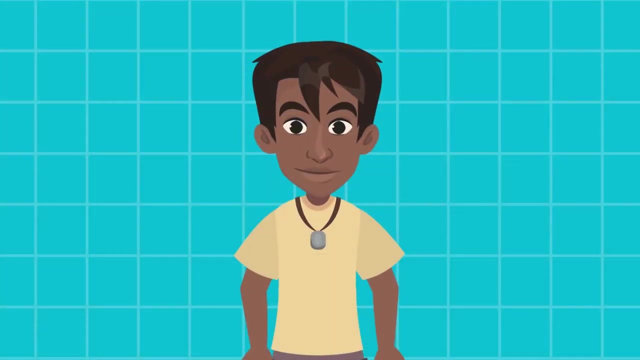 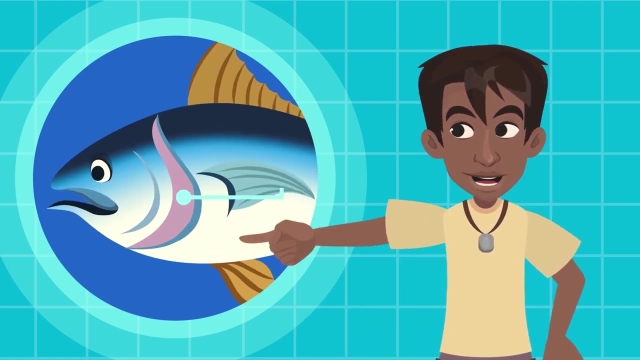 and seas are saltwater habitats. there we find a great diversity of animals like whales, sharks, coral or seahorses. there are also plants that grow in the sea, like seaweed. in aquatic habitats. the living beings have adapted to carry out their activities under the water. an example would be fish bronchia that. 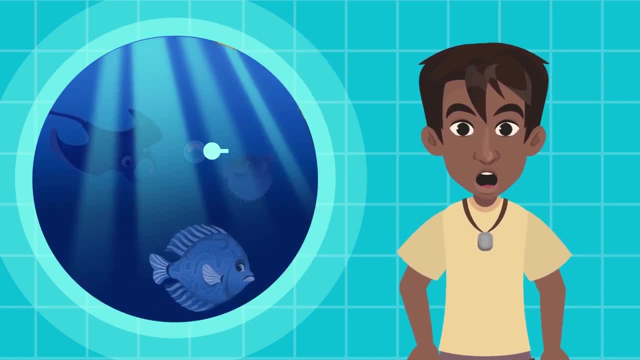 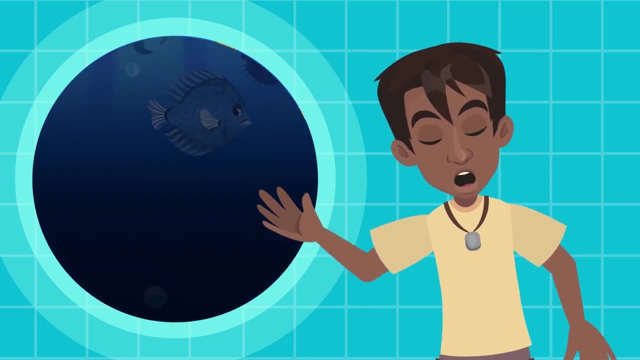 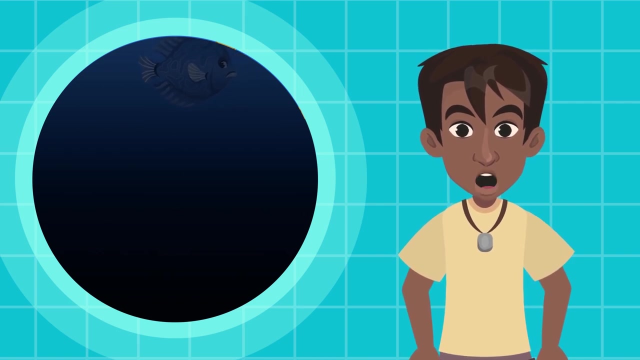 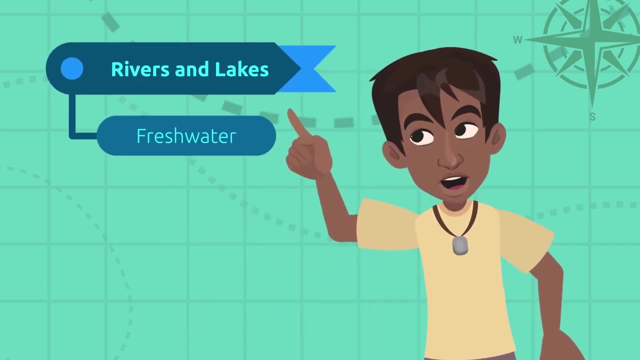 allow them to breathe. underwater in these habitats, light is a very important resource too, and sometimes, due to contamination, it cannot reach deep enough to the bottom of rivers, lakes or oceans, leaving the living beings without an essential resource. today we learned that aquatic habitats are distinguished as freshwater rivers and lakes, and 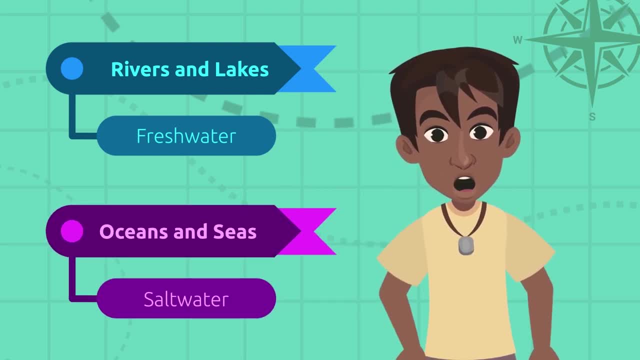 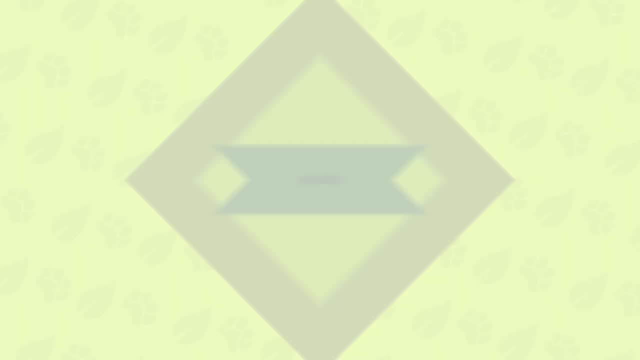 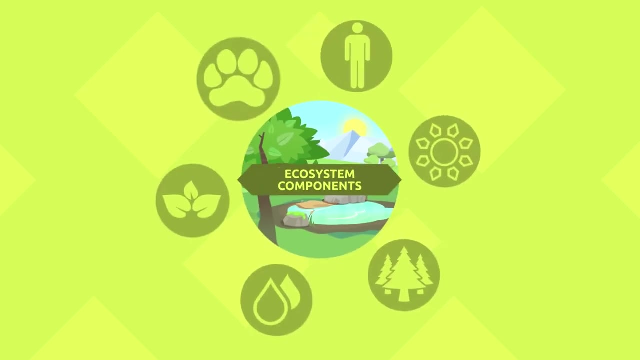 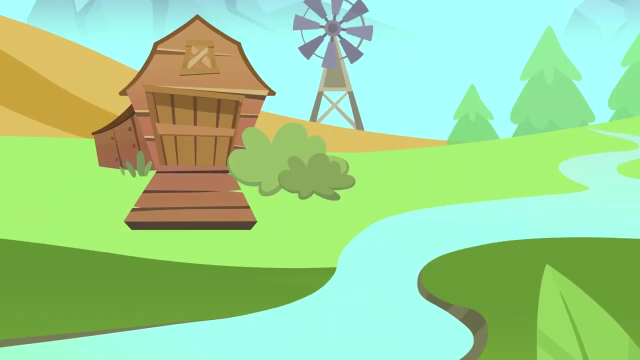 saltwater, oceans and seas. that was all about habitats. see you soon. today, we're going to learn what an ecosystem is, its components and the different types of ecosystems found on earth, ready to learn about them. an ecosystem is the community of the living organisms and the natural resources of 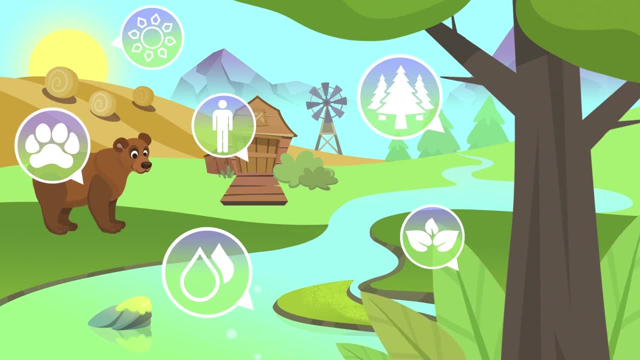 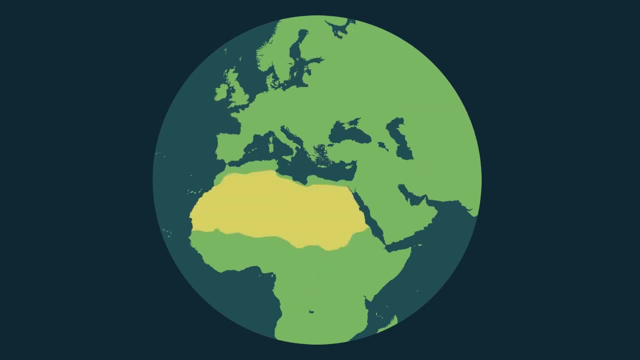 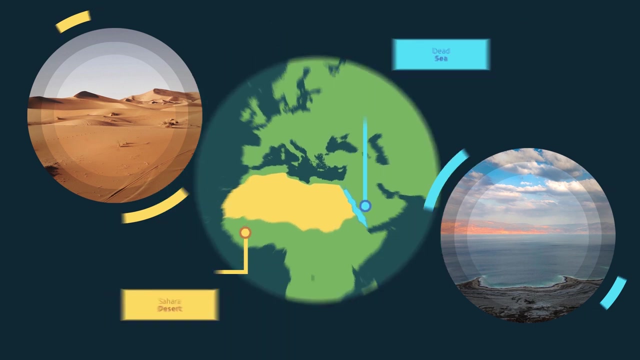 the environment in which they live. ecosystems are found in different parts of the planet, and they can be found in different parts of the world, such as the ocean. they can be very big, like the Sahara desert, or much smaller and circumscribed, like the Dead Sea. but how do we identify ecosystem coverage? the 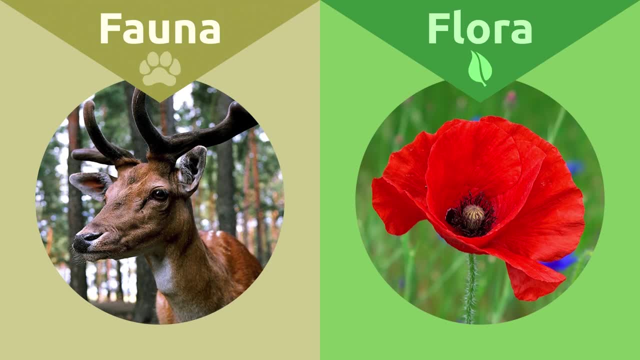 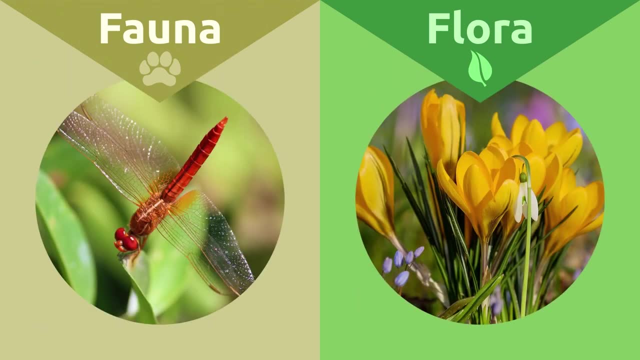 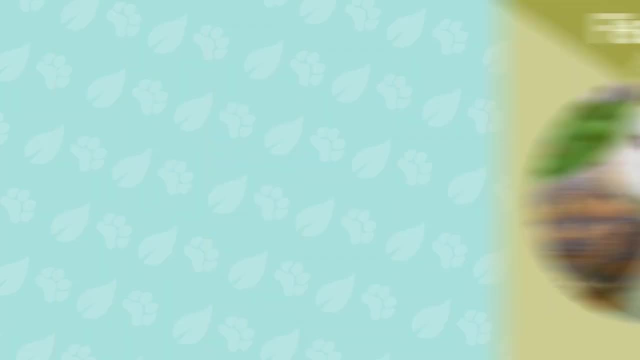 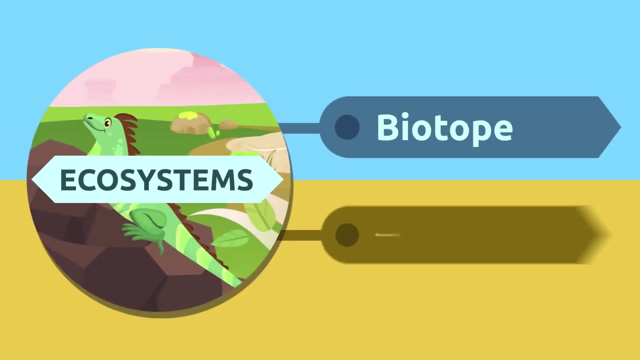 flora and fauna of each ecosystem have adapted to live according to the characteristics and resources of their surroundings. the interaction among them defines the ecosystem and its coverage. that's why there are so many types of ecosystems. ecosystems consist of a biotope and a biosynosis. let's see what they are. the 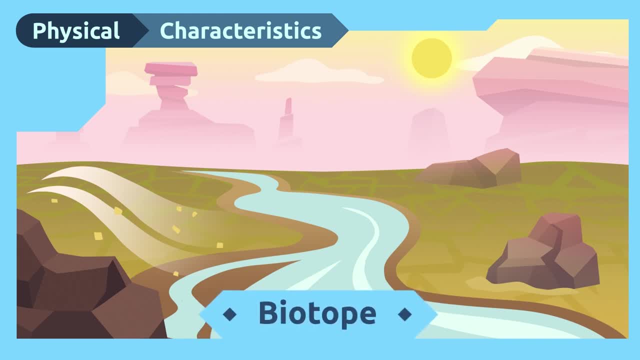 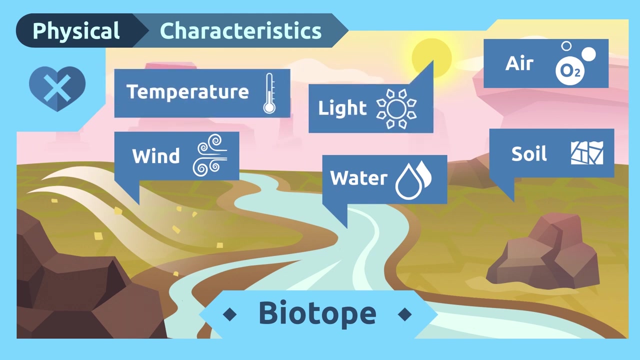 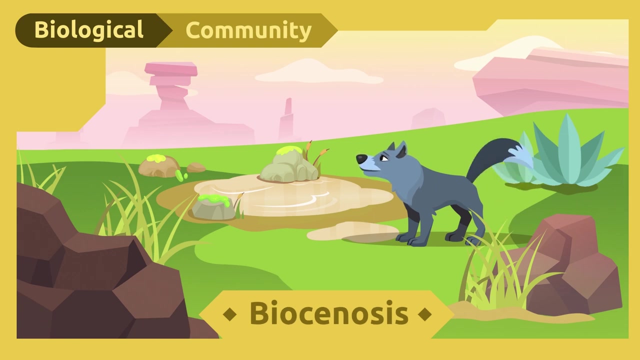 physical characteristics of the surroundings are called a biotope. these characteristics include non-living elements like the soil, the water, the air, the wind, the light or the temperature are called buccaneer 1. the biological community that lives in those surroundings is called a biosynosis, that is to say the living beings that 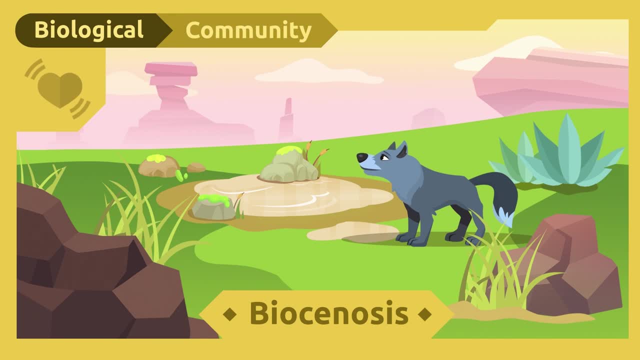 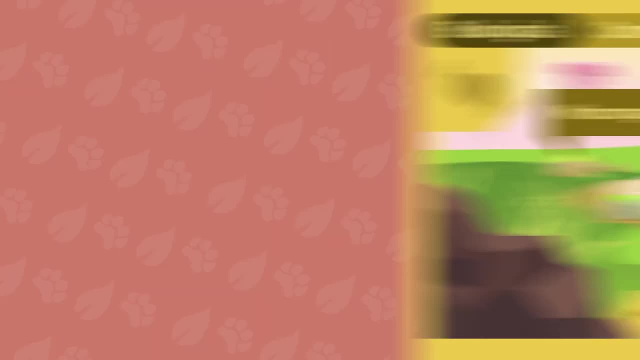 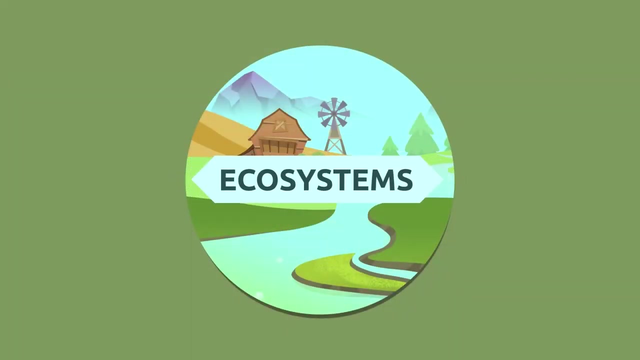 live in a physical area. among the living beings that make up the communities in an ecosystem, we can find microorganisms, plants and animals. we distinguish between two types of ecosystems. the ответ can be by the number of living being in one of ecosystems: natural ecosystems and artificial ecosystems.